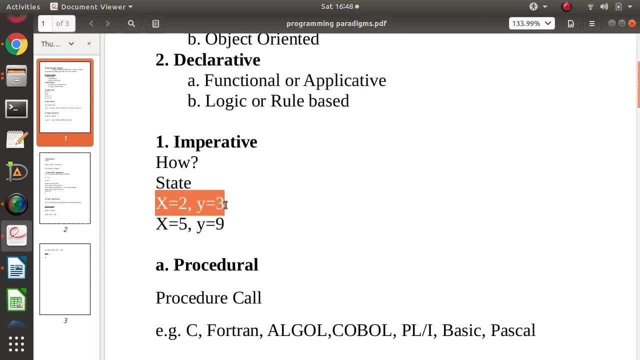 Suppose we have two variables, x and y. So at some time, suppose x is equal to 2 and y is equal to 3.. This is the state. So at a particular time instance, whatever the values are saved or allocated to, the variable is called as state at that particular time. After some time, 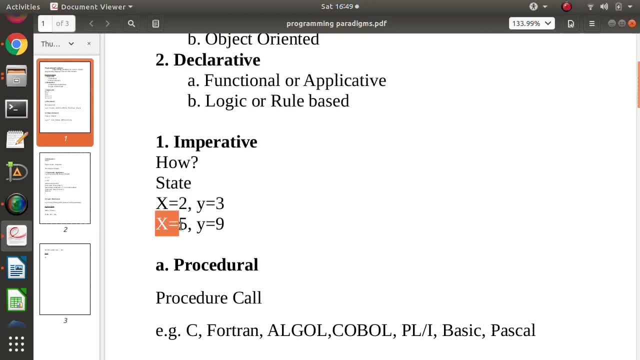 suppose x is get allocated to 5.. Now x is equal to 5 and y is equal to 9.. So this is the state at that particular time. After again, after some time, suppose value of x will get changed, value of y will get. 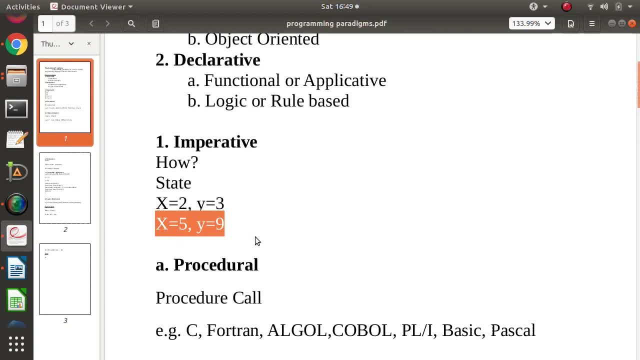 changed, So that will be the state at that particular time instance. So this is how, as time passes, state also get changed. Imperative programming paradigms focus on how state get changed, So it mostly focus on state changes, While in declarative programming paradigm 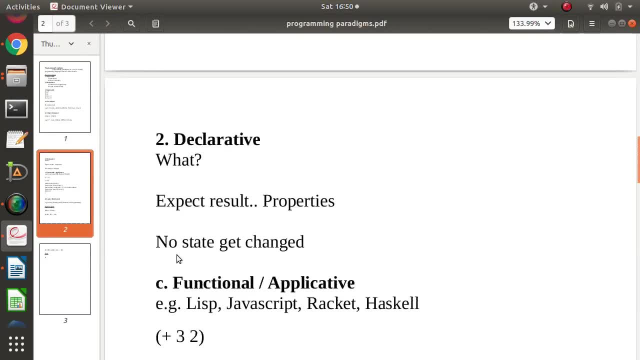 there is no state, get change. So it not change any state. It takes inputs and this declarative programming paradigm focus on what, What in the sense, what result you are expecting, What are the properties of result that you are expecting? So here we are not focusing. 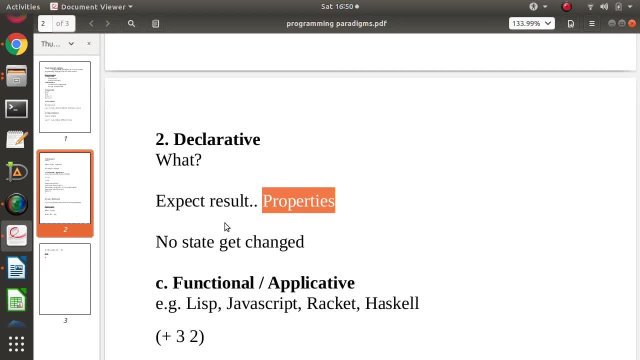 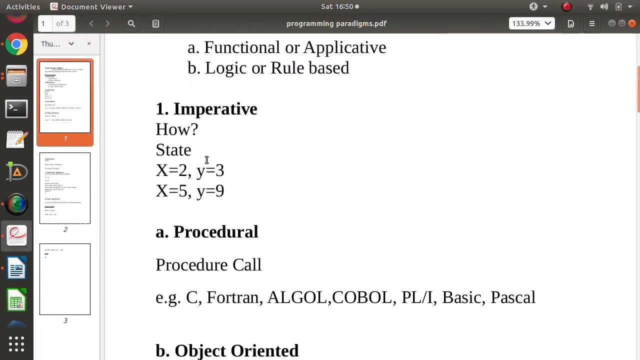 on any state change. Here we focus on the output And while getting output, we expect result or we expect some properties from the result. So, mainly declarative programming paradigm, we focus on what, What type of result you want, While in imperative programming paradigm we focus on how we get the result, how we 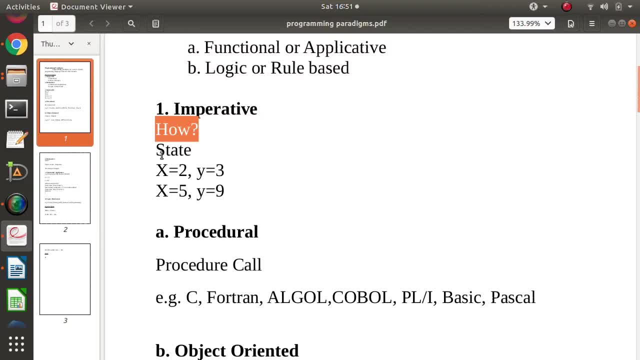 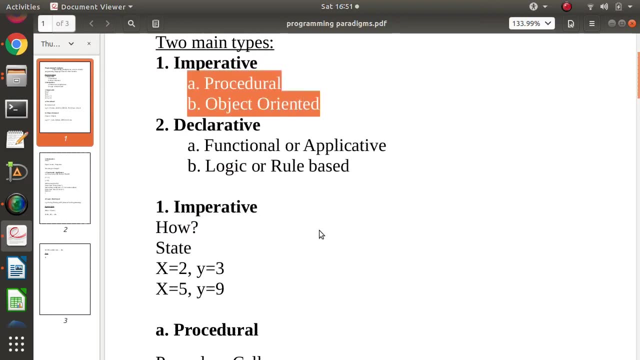 get the final output. So for that state get change, while in declarative programming paradigm there is no state change. Imperative programming paradigm: Again, we have two types, as we have seen here. One is procedural and another is object oriented. Now look at this. 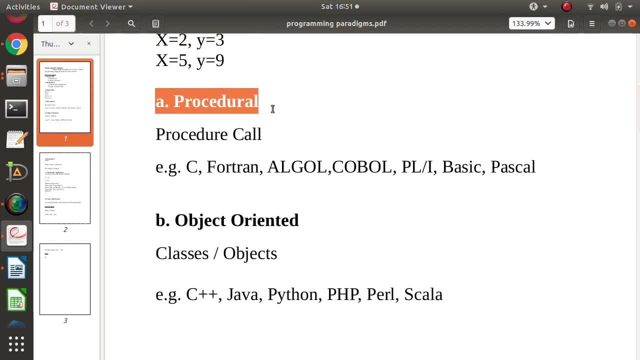 So what do you mean as procedural programming paradigm? So one thing is a special here, That is the procedure. Procedure means a set of statements or sequence of statements that becomes a procedure, or we can also call it routine. So set of statements is called as a procedure and whenever we require we make a call to. 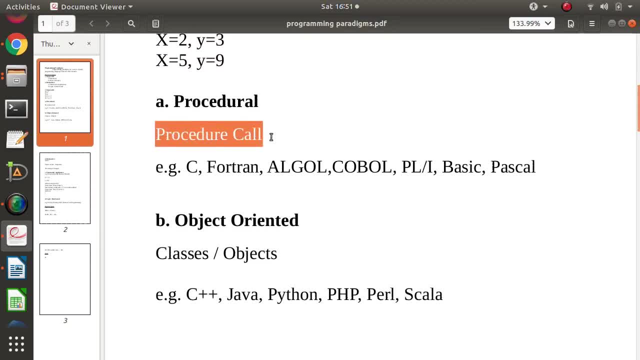 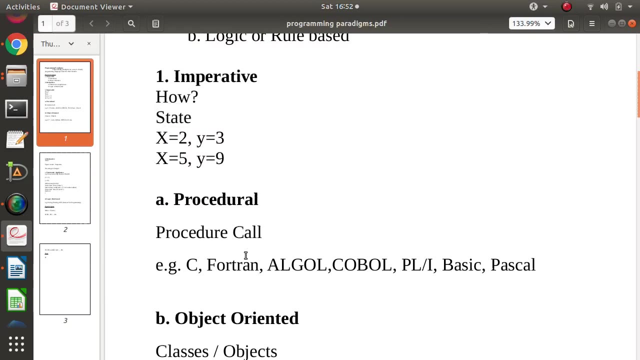 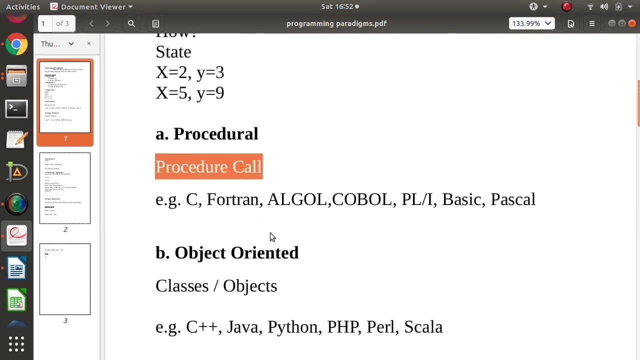 that procedure we call it procedural call. So procedure is nothing but a set of statements and the set of statements changes state. This procedure set of statements changes the state and whenever we require that we make a procedure call. So such kind of programming paradigm is called as procedural programming paradigm. 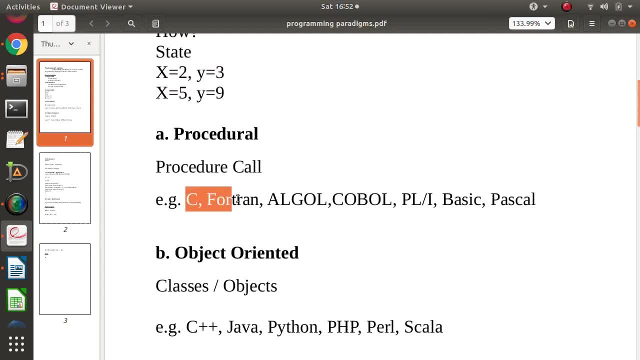 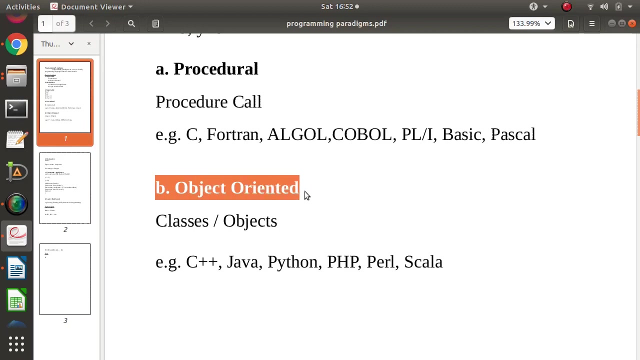 Example of procedural programming paradigm is C, Fortran, Algol, COBOL, PLI, Basic And Pascal. These are the programming languages which are which follows procedural programming paradigm. Now see second type in imperative programming paradigm is object oriented programming paradigm. 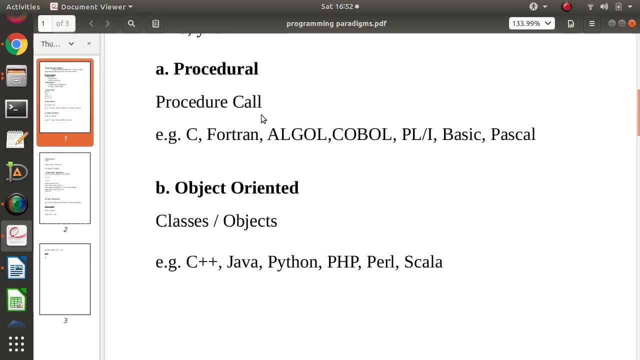 Now see, in procedural programming paradigm we were writing simple set of statements, right, a collection of statements. But that was boring. right Then it was thought: why programming cannot be done interesting, why it cannot be made more realistic? So what is around us? around us, everything are all objects. 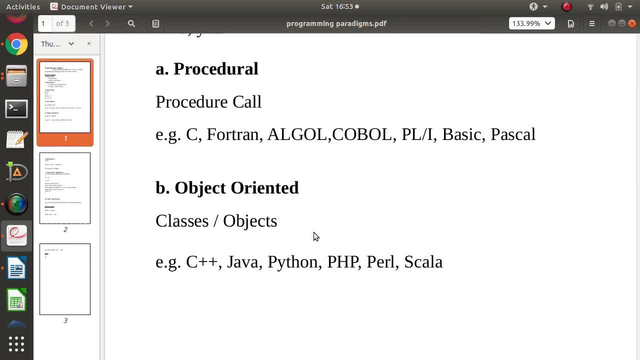 So, for example, we are surrounded by the objects. only Example: if you take fan, fan is an object, right, So it has some parameters. For example, It has a number of blades, It has color, Then it has some voltage. It requires some watts. 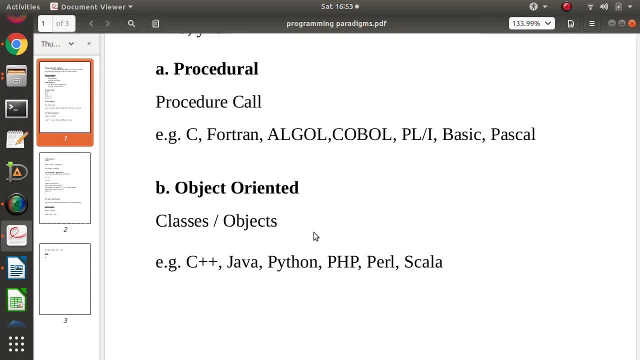 So these are the parameters for that particular object. Now, what operations we can perform on this object, on this fan. We can switch on, We can switch off, We can change the speed. All these are the operations which can, which we can perform on the fan. 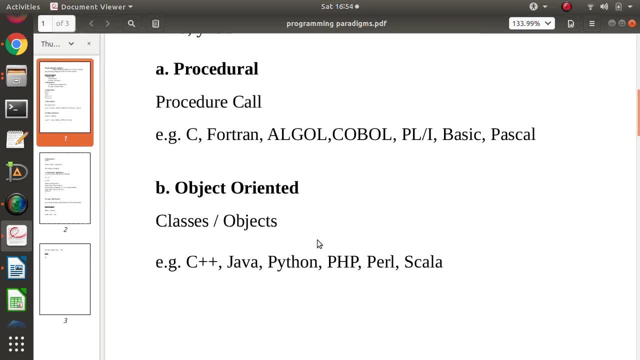 So what are the parameters Of this object- We call them variables- And what are the operations which we can perform on this parameters or on this object? We call them functions. When variables and functions combine together, it becomes class. So there is a concept called encapsulation. 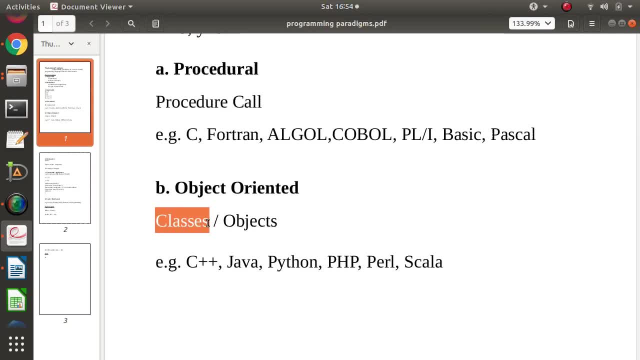 So encapsulation means we are combining these variables and functions together and we get a class And instance of this class function. We call it class, We call them objects. So suppose in a classroom where I am sitting, suppose there are five fans. That means there are five instances of class fans. 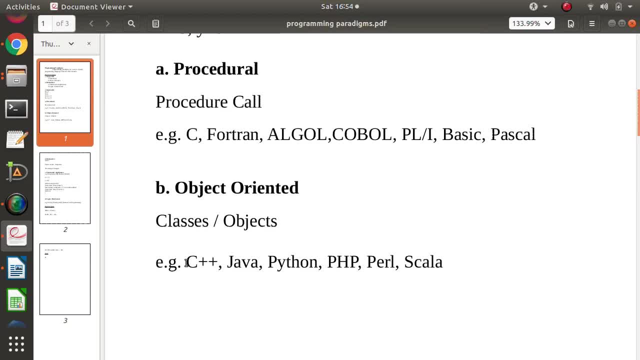 Now see, these are the different types, or these are the different programming languages which support this object oriented programming paradigm: C++, Java, Python, PHP, Perl, Scala- All these are the different programming languages which support this object oriented programming paradigm. All these languages follow object oriented programming paradigm. 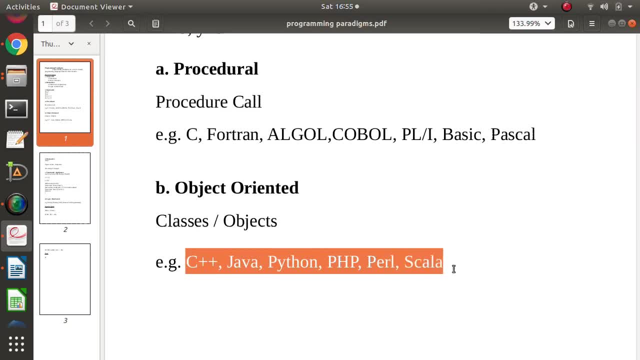 All these are the examples of object oriented programming paradigms. All these languages follows object oriented programming paradigm. There are various concepts which define this object oriented programming paradigm, For example polymorphisms, inheritance, data abstraction, etc. Polymorphism means multiple forms. 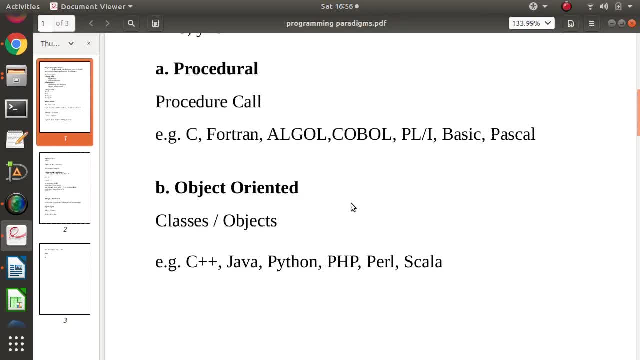 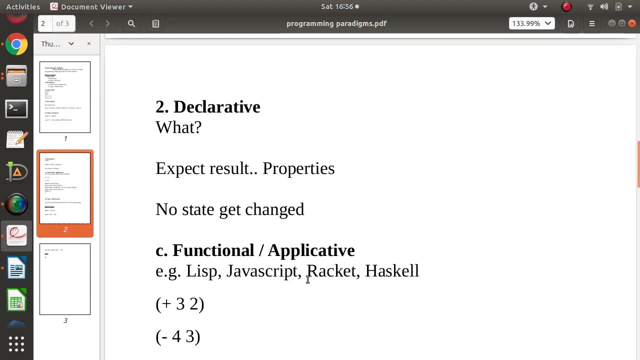 Single things have multiple forms, While inheritance data, While Inheritance means reusing classes, so that we call Inheritance. so this is called as Object Oriented Programming Paradigm. Now in Declarative Programming Paradigm, again there are two types, so Functional and another. 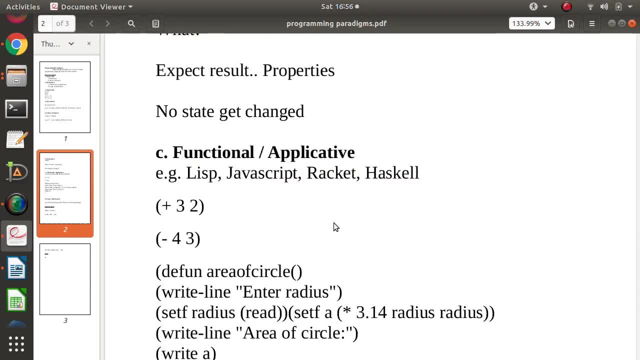 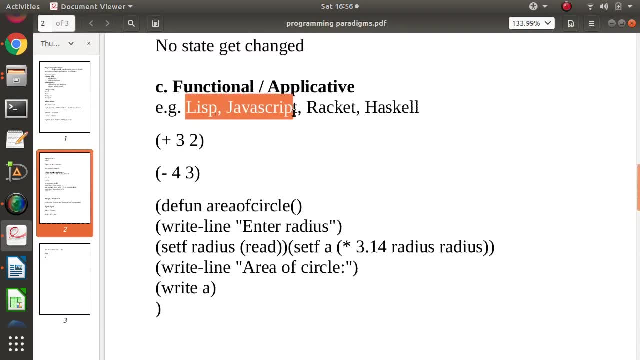 is Logic, so Functional Programming Paradigm. examples of Functional Programming Paradigms are Lisp, JavaScript, Racket, Haskell- all these programming languages follow Functional Programming Paradigm. So what do we have? Functional Programming Paradigm. Here all statements are written as a Functional Call. 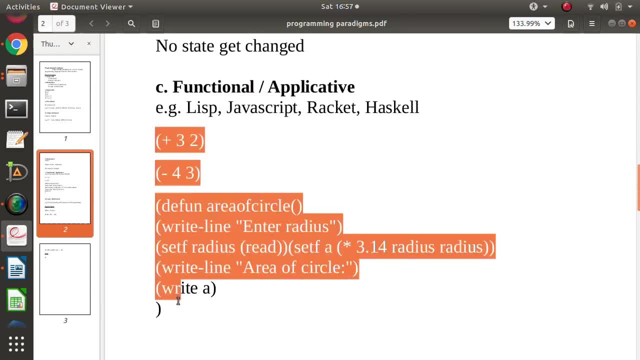 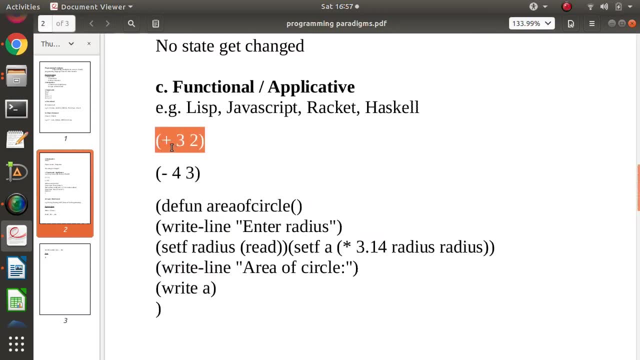 For example: see: these are the statements I have written from the Lisp programming language. Now look at this is Addition. So for Addition, Again Here we are calling a Function Plus. So here Addition Plus is a Function Minus 4, 3. this is also a Function for Subtraction. 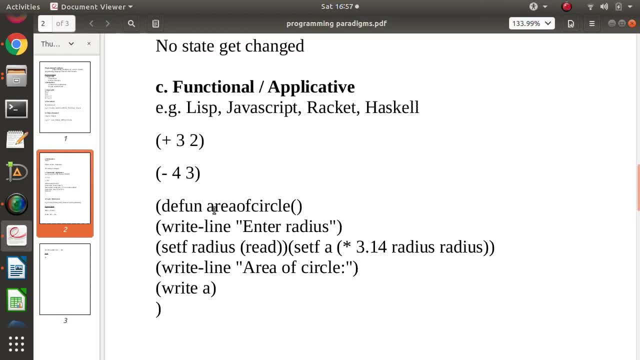 So every statement here is a Function Call Even to define a Function. we use one Function, So Define is a Function which is used to define another Function, Area of Circle. So example I have taken here: Area of Circle, So to define a Function. 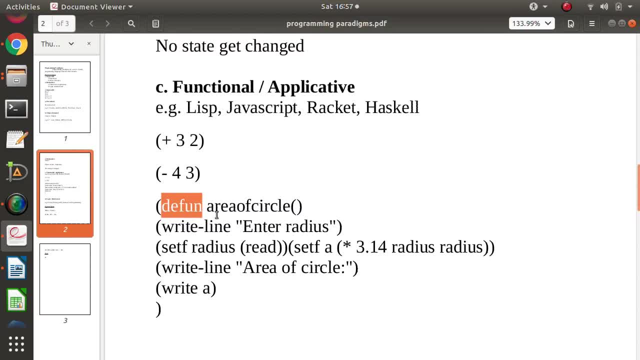 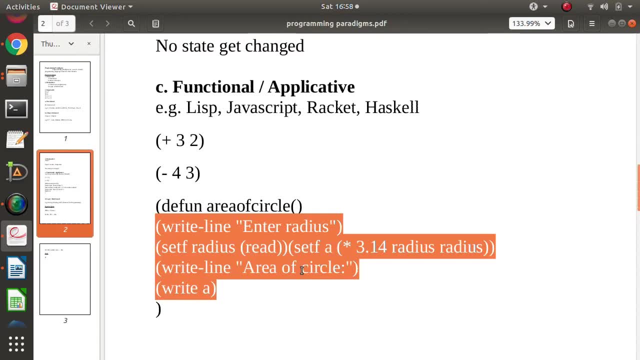 Again, we require a Function. So these are the statements in this Area of Circle function. So all these are a Function Call. So WriteLine Setup, WriteLine, Write, all these are the Function Call. So in Functional Programming Paradigm, all statements are the Function Call. 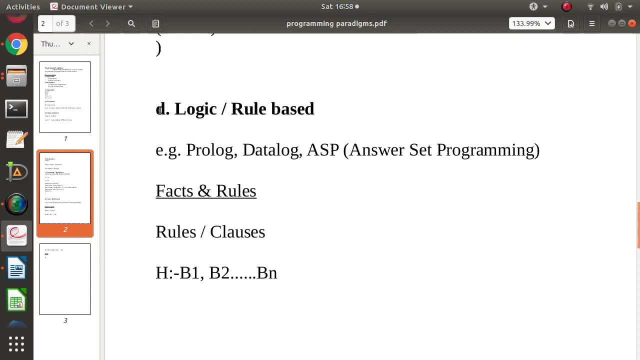 Now we will see another programming paradigm, that is Logic- All Rule Based Programming, Paradigm. So again it is the Addition. So again it is the Addition, So the Addition: All statements in Logic, All Rule Based Programming, Paradigm, rules such as Prolog, Datalog, ASP. 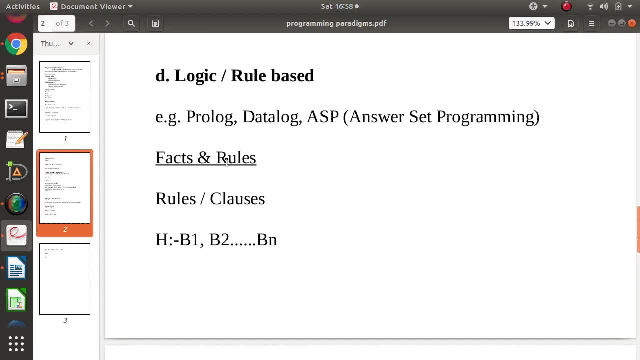 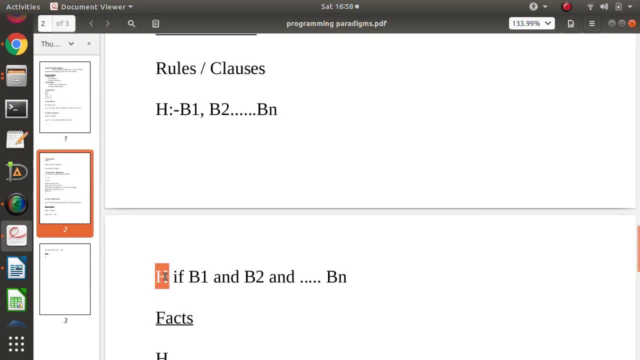 kee here, Here, every statement in Logic, All Rule Based Programming Paradigm is Facts and Rules. So let us see this: Facts and Rules. So the rules are written like this. So what do you mean by this? h is true if b1 is true and b2 is true, and all these conditions. 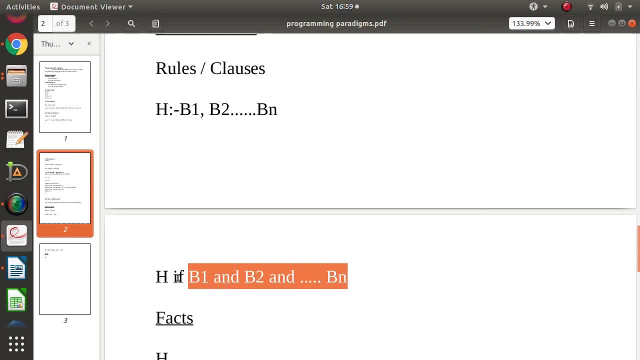 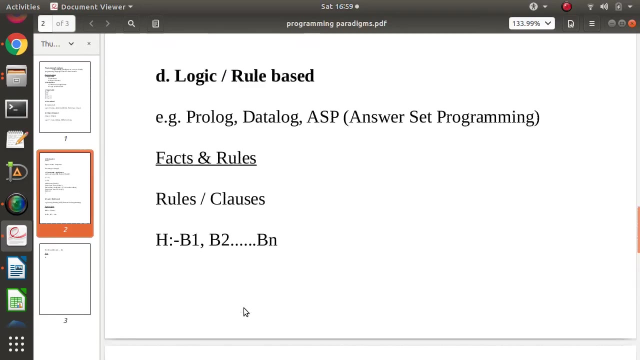 are true Means if b1,, b2, bn- all these are true, then the statement h is true. So these statements are called as rules, that is a clauses, and facts means simple statements. So whenever all the statements in any programming language are written in the form of facts,